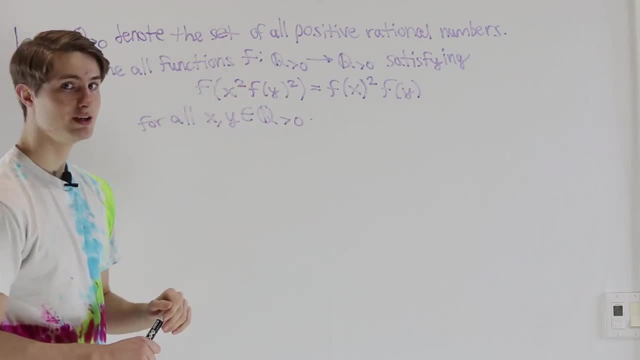 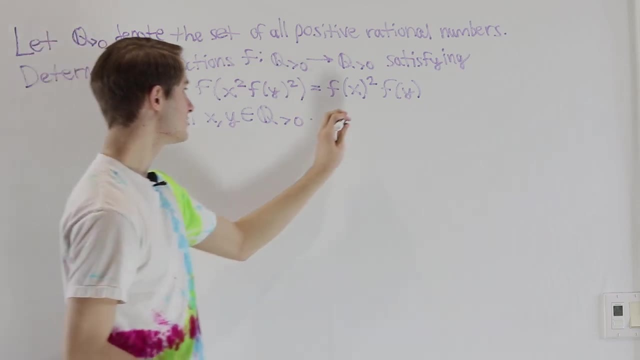 are squared. All we need to do to make this perfectly symmetric is to make both of these look the same. Right now we have x and then f of y. So what if we just said: Let's let x equal f of a for some number a that we're? 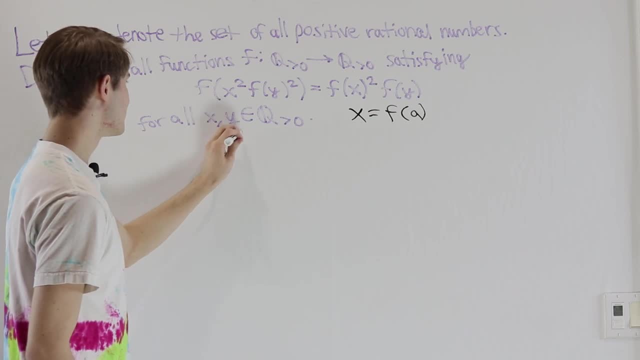 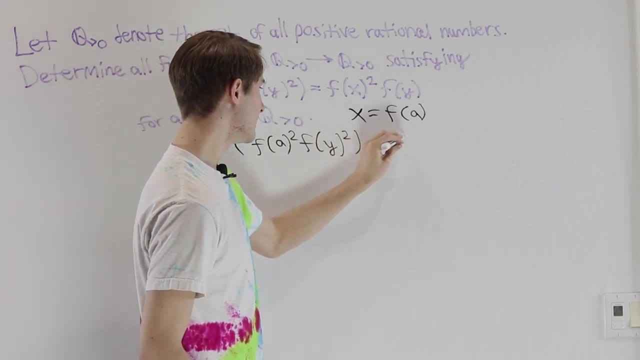 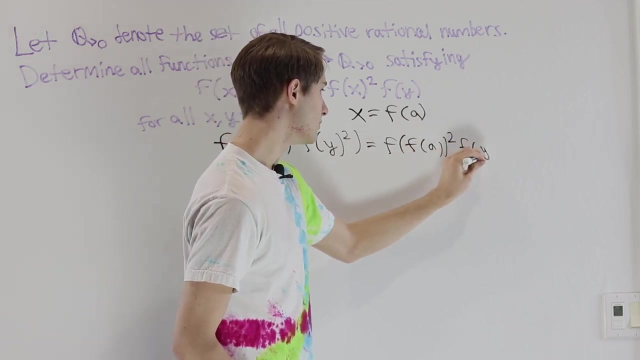 defining. now, If that's true, then what we get is f of f of a squared times f of y, squared equals f of, in this case, x is again f of a equals f of squared times f of y. Now we have exactly that symmetric thing that we're looking for. 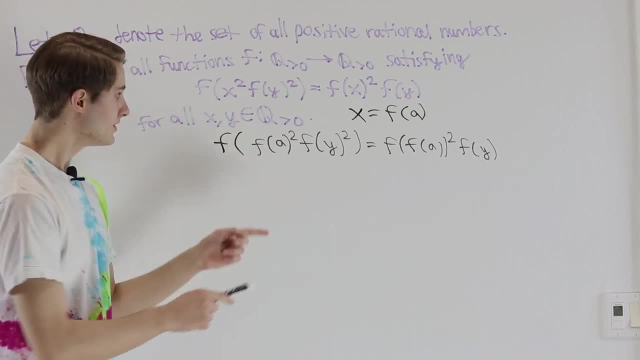 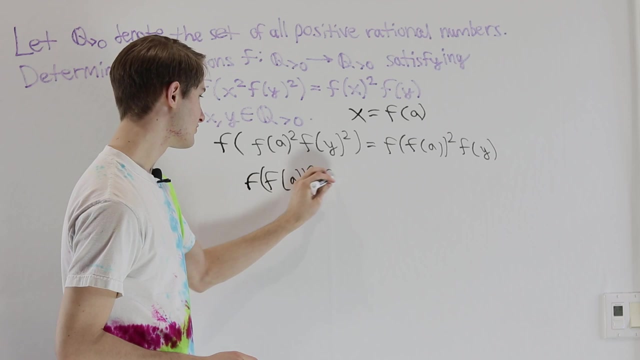 And now what we can do is, because this is symmetric, we know that this output right here is going to be the same if we flip the values of a and y, which means that this function here f of f, of a squared f of y- well, that's equal to this. So if this part, this expression, 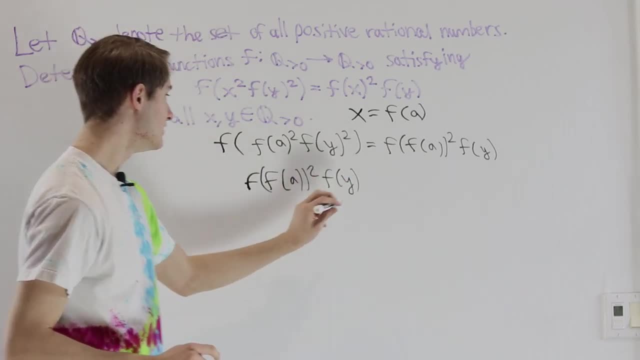 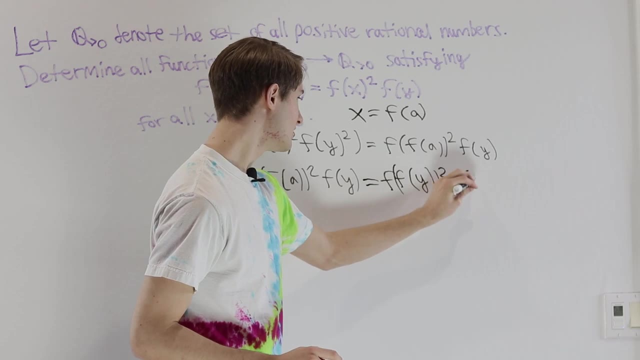 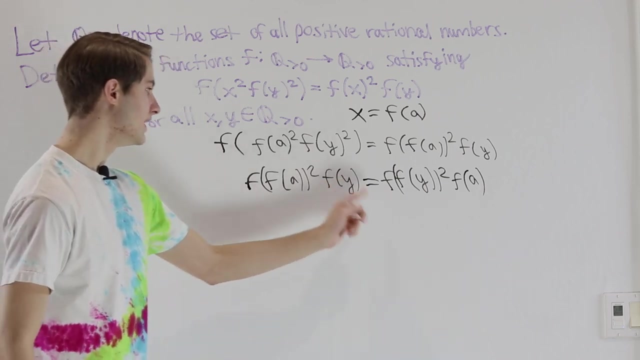 here stays equal when we switch a and y. this also has to stay equal when we switch a and y. So we know that this equivalence has to be true. f of f of a squared times f of y must equal f of f of y squared. 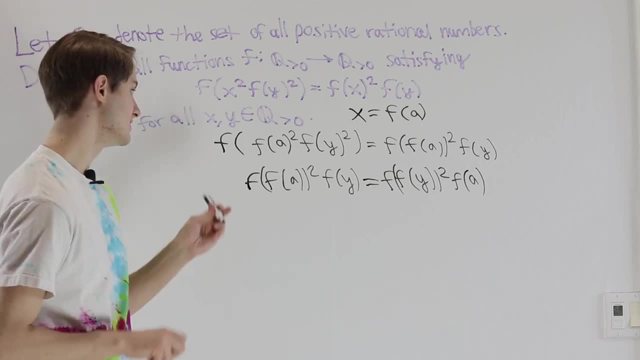 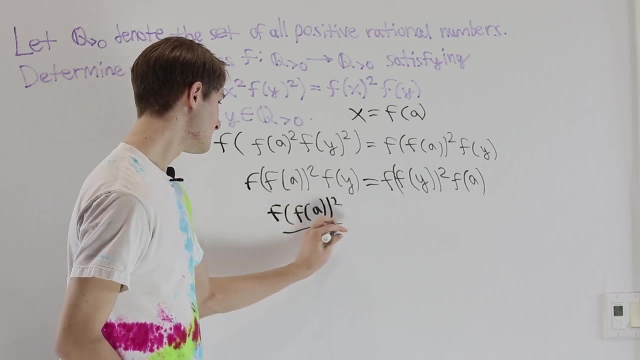 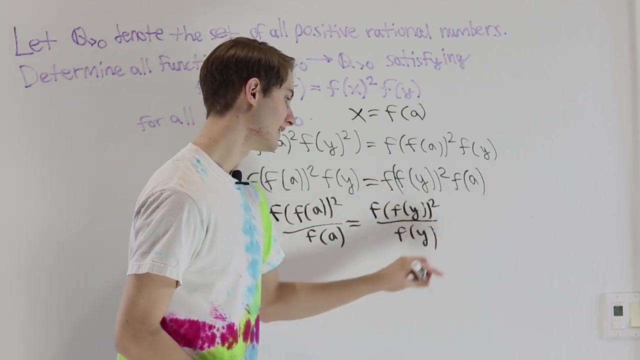 Now let's isolate the variables on each side. So on the left side, we're going to get f of f of a squared over f of a, and on the right side, f of f of y squared over f of y. Aha, Now we have some more symmetry, and the reason this symmetry is very helpful is: 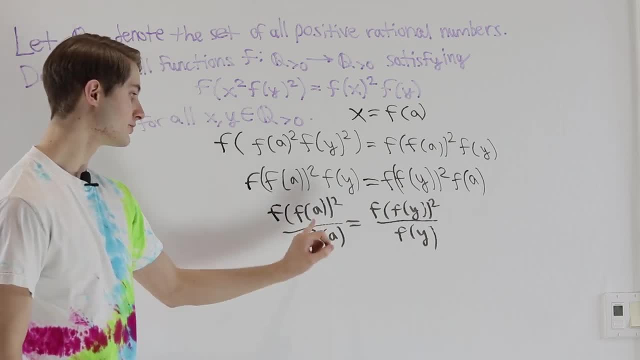 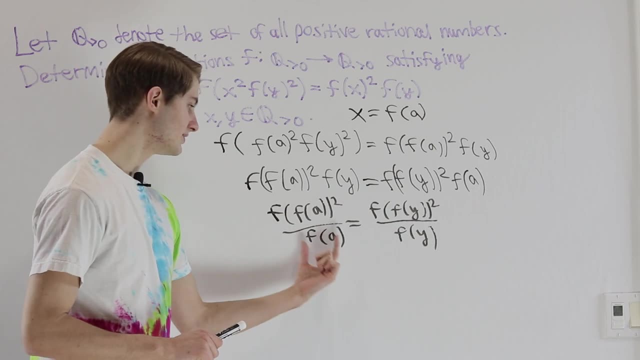 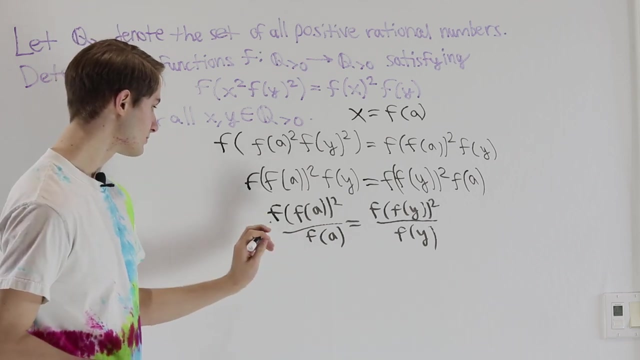 because we know that this expression is the same for two different inputs, a and y, And because we can pick a and y to be whatever we want, that means that this expression has to be the same for every single possible input: a or y. So this expression that we have right. 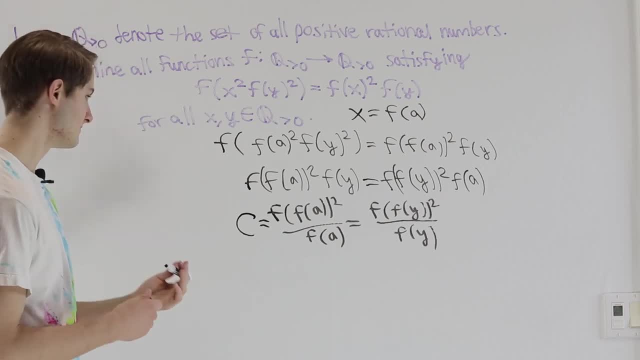 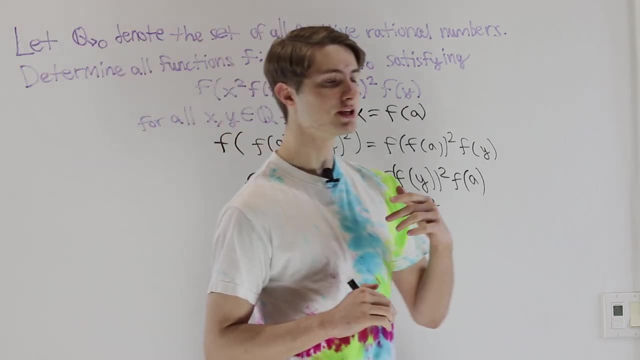 here must be equal to some constant c. Now let's see if we can find another instance of symmetry in this equation that we have here, something that will get the two sides of our equation to look more similar. Well, right now we have all the functions on the. 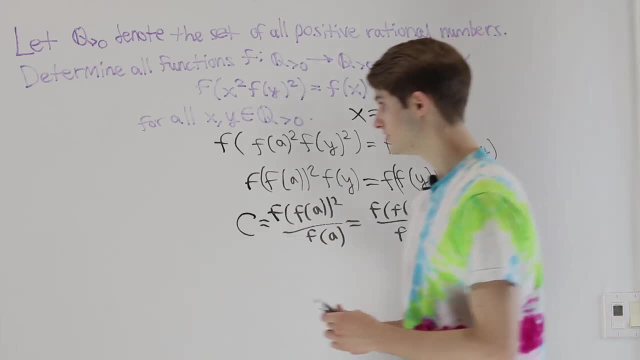 right side of the equation. So we're going to have f of f, of f squared over f, of a squared over c, squared times, c squared. Now how do we try and write that? Well, let's try to do some more cooled down equations, but first of all let's assume that we've got the 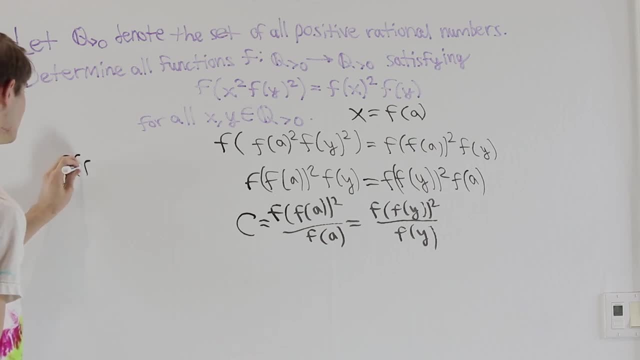 same equation on the left side. So let's deal with that first. If we multiply by f of a on both sides, we're going to get f of f of a squared equals c times f of a. Now notice that we have c only on one side of the equation. Well, right now, if we divide by c, then we're. 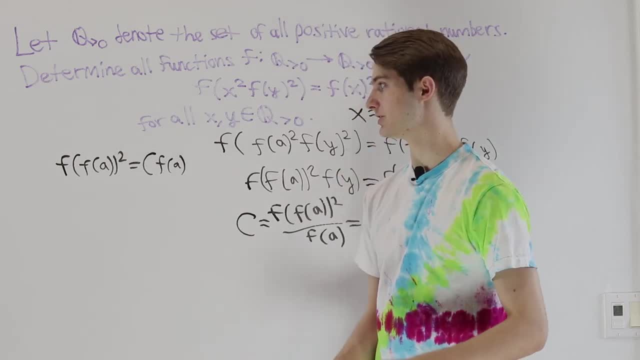 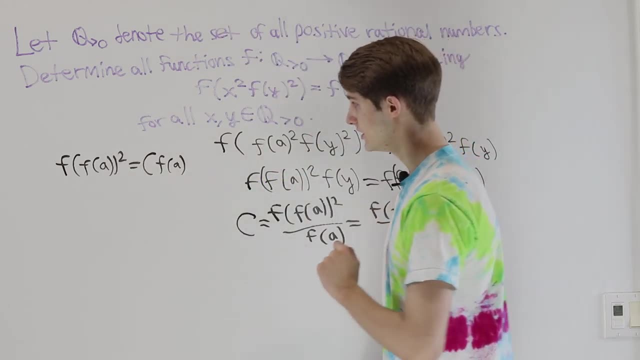 just going to move it from one side to the other side, but that's still not symmetric. So we want to find something else that will let us put c on both sides of the equation To do that. notice this: On the right side we have this function thing to the first power. 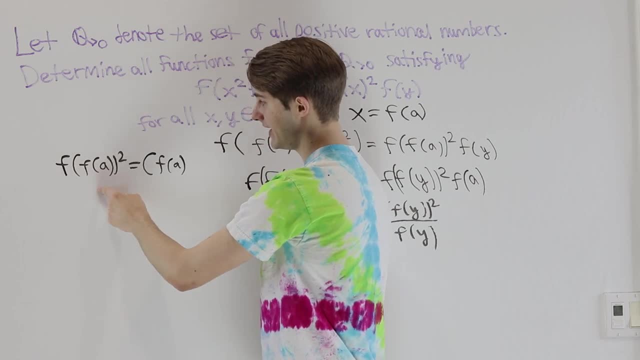 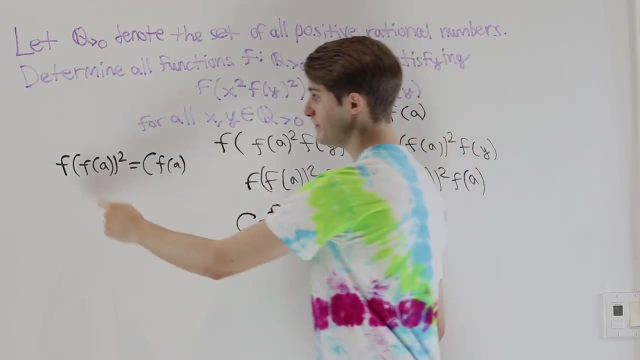 But on the left side of our equation we have f of f of a and then squared. So what if we'd put divided by c squared on the left side, so that it matches with the square that we already have Now? in order to do that, we would have to divide by c, squared on both sides. 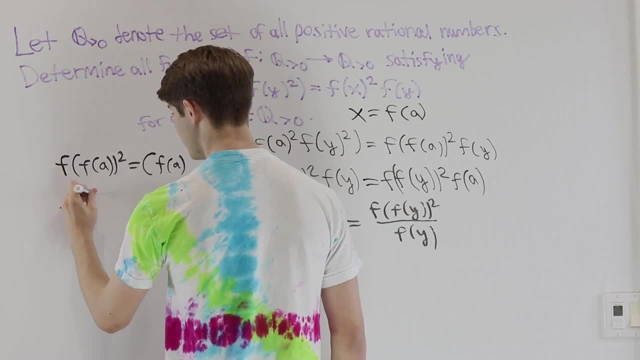 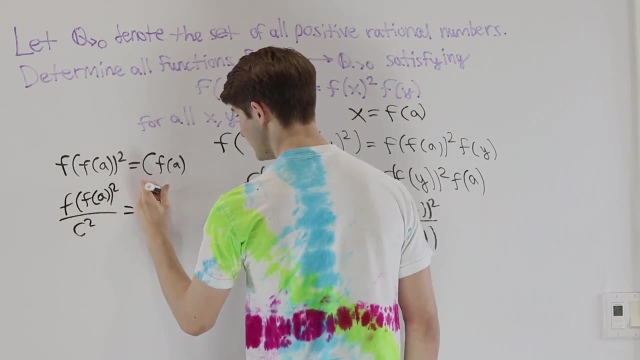 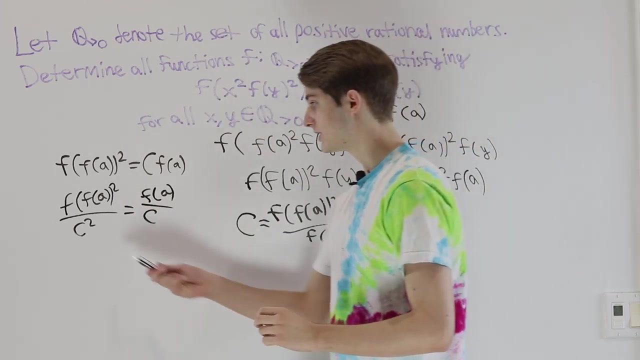 So let's see what happens. when we do that, We're going to get f of f of a squared over c squared equals f of a. and then when we do c over c squared, that's going to leave us dividing by c And now realize that because we divided by c squared over here, we were able to keep the c on the right side. 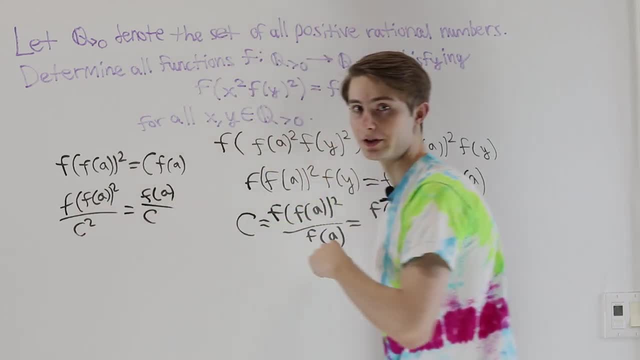 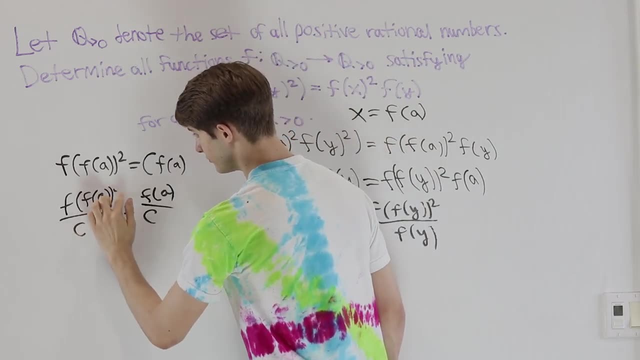 And now we just have squares on the left and the first power on the right, So this is looking much more symmetric. The last thing I'm going to do is factor out this power of 2. From both of these parts on the left, so that we take it all the way to the outside. 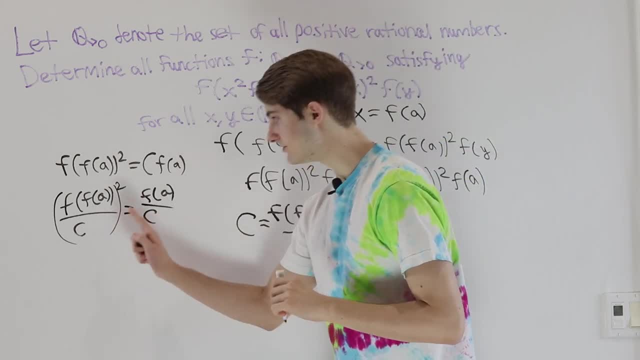 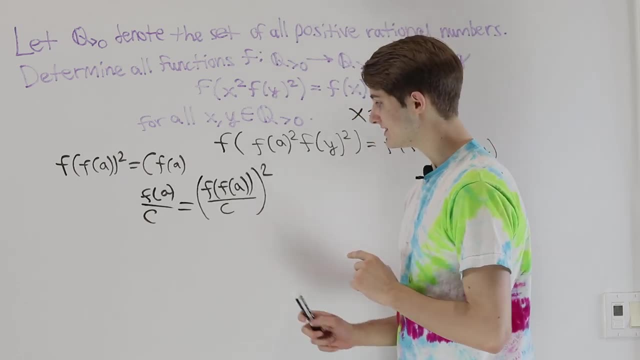 f of a over c equals f of f of a over c squared. So now that we have this nice symmetric equation, what you might notice is that this is a very interesting equation, So we're going to try to have some fun with it here. 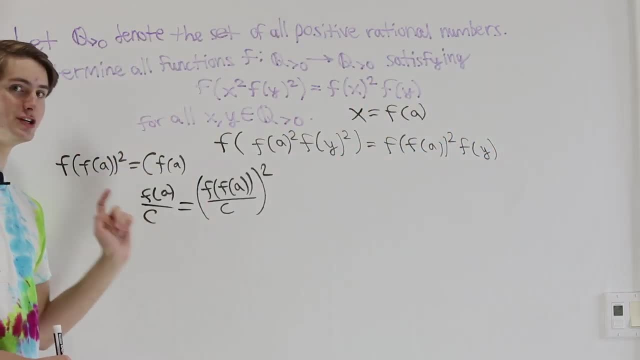 Let's do some experiments and see what we can figure out using just this equation. First of all, notice that on the left side we have f of something over c, And on the right side, inside of our parentheses, we have f of something over c as well. 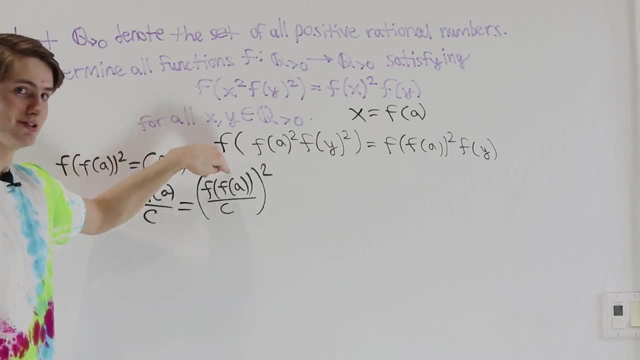 It's just that on the left the input is a and on the right the input is f of a. But we could easily apply this equation to the right side here, And what that would leave us is that f of f of a over c squared. well, that's going to equal. 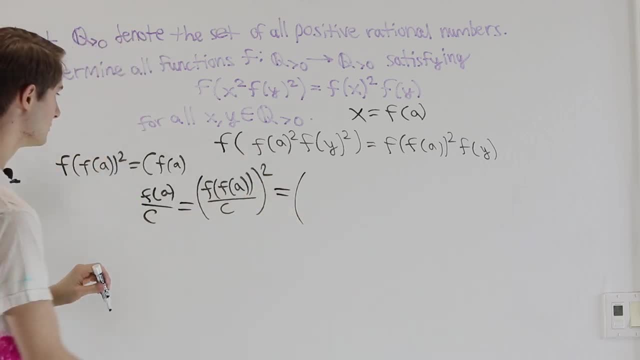 let's think about what happens to the inside of these parentheses. Think about this as f of something over c. But we know from this equation that f of something over c is going to equal f of f of that something over c, and then squared. 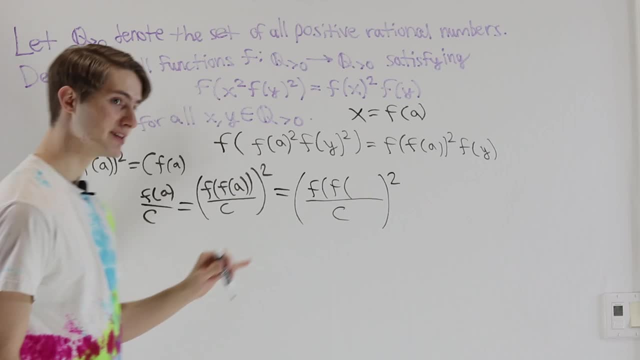 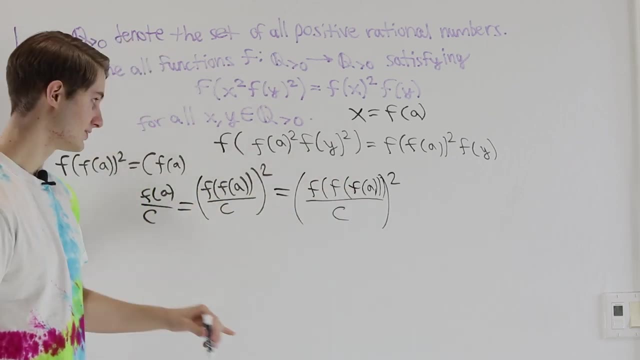 But this time what we have inside of that parentheses, instead of a, is f of a. So now we've gone from two to three iterations And then from here we have to remember that square that we already had in that original expression. So suddenly, instead of having f of f of a and squared, 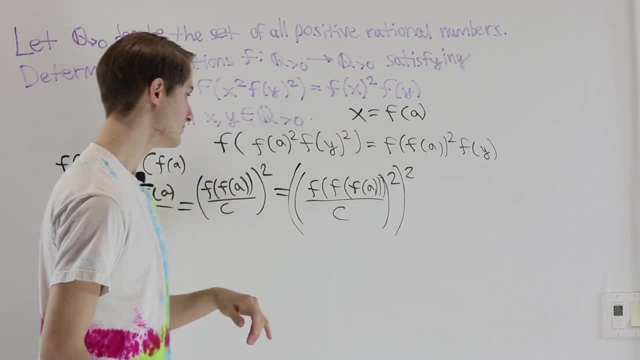 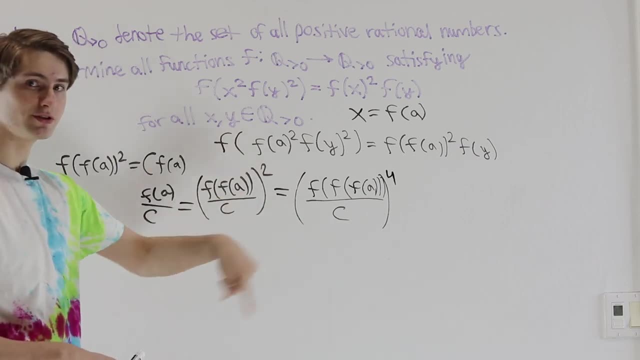 we have three iterations of f, and then to the power of two times two, which is equal to four. And we could keep applying the thing that we just did over and, over and over again to this input, Because now, instead of the inside of our function being f of a, 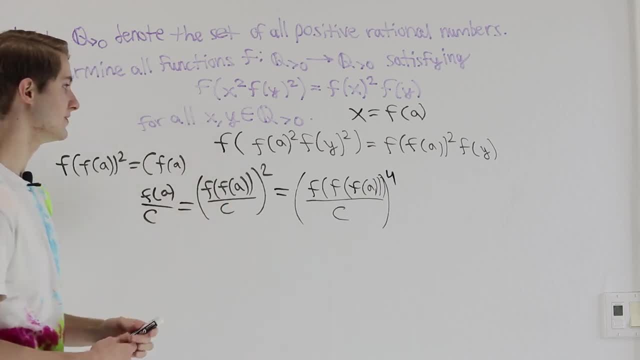 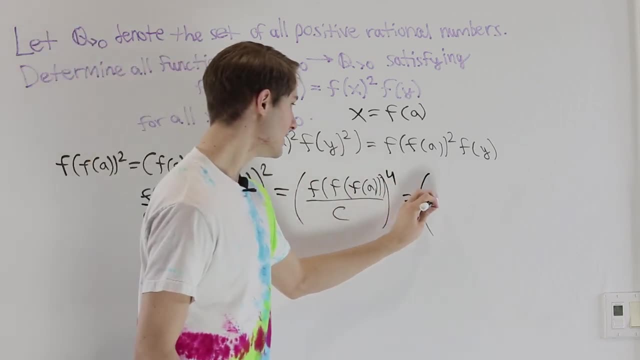 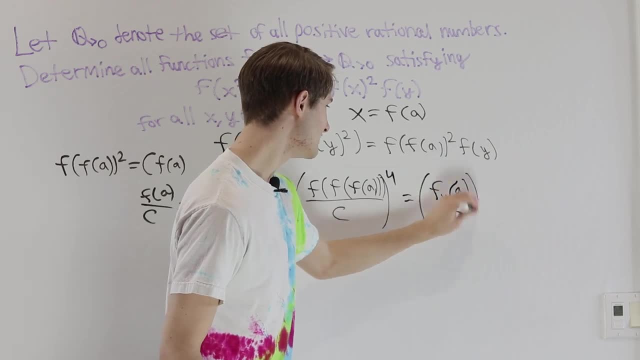 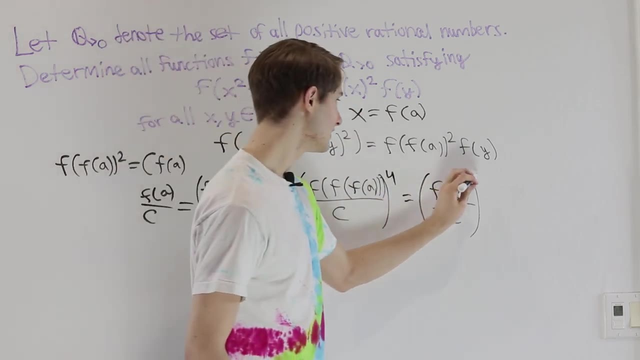 So f sub four of a over c. Well, first we had squared, then we had to the power of four. If we squared it again, we would get the power of eight. After that we get the power of sixteen and thirty-two, and so on. 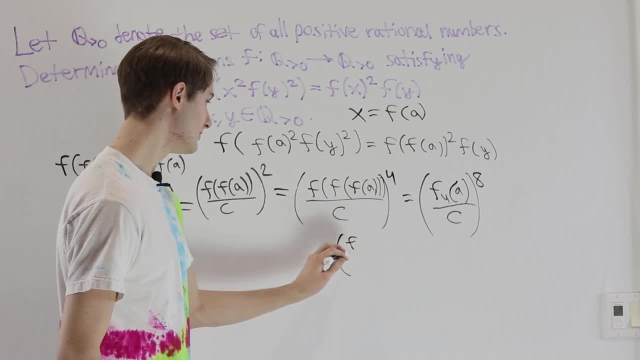 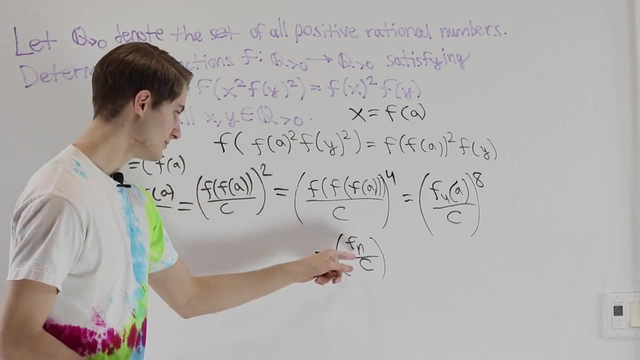 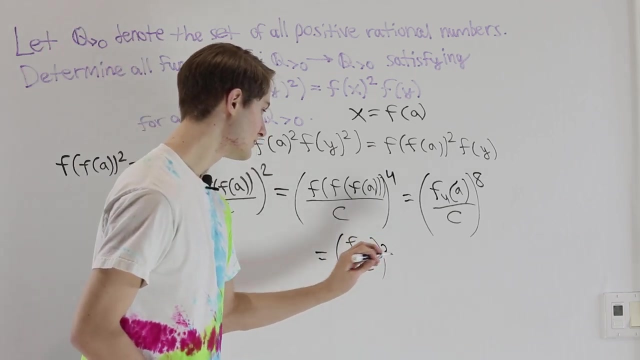 In general, this is going to equal f sub n over c. So we've done n iterations And let's think about, based on this number n, what power are we raising this expression to? Well, we know that it's going to be some power of two. 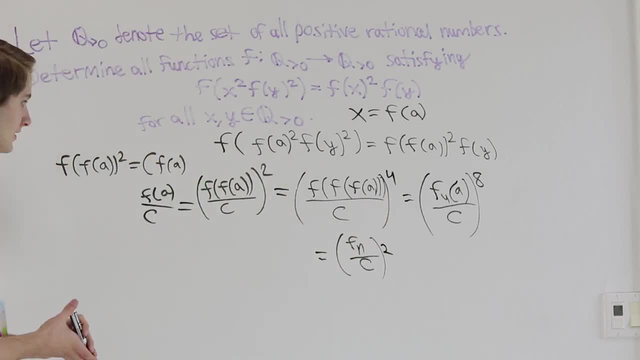 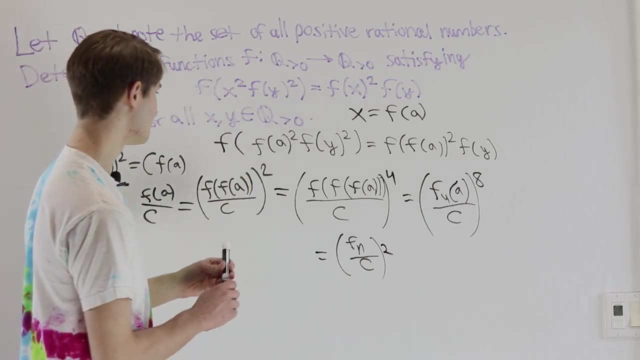 It's going to be two to the something. But let's figure out what that is. When n is equal to two, f of f of a, we have squared, or two to the first power. When we have n equals three, it's two to the second power. 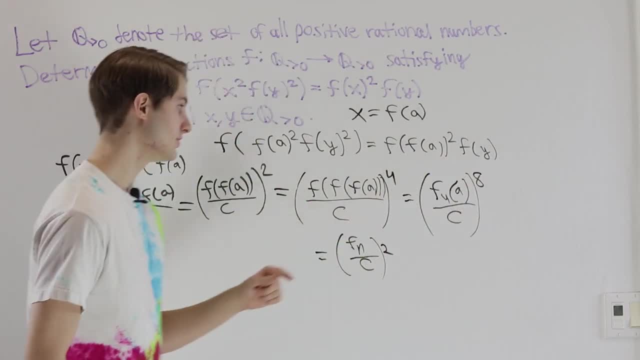 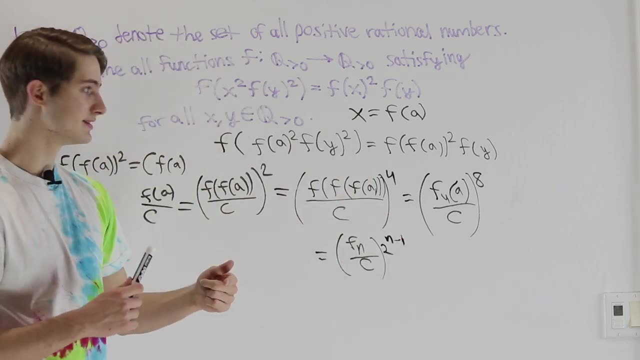 When n equals four, it's two to the third power, Or, in general, it's going to be two to the n minus one, Because that power is always one less than the number of times we apply the function. So this expression that we have right here, 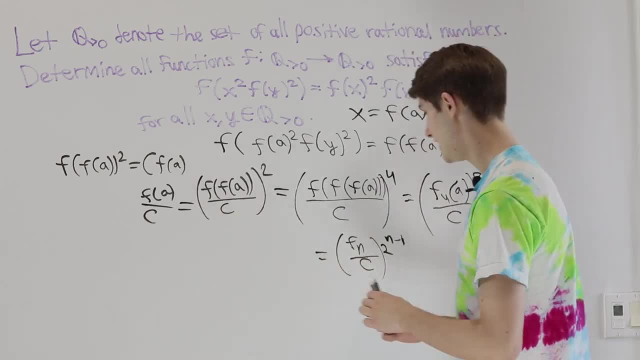 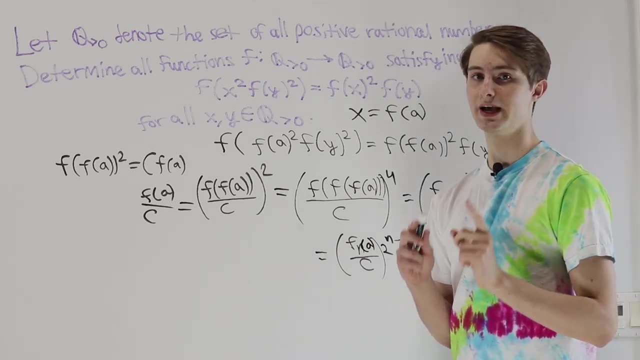 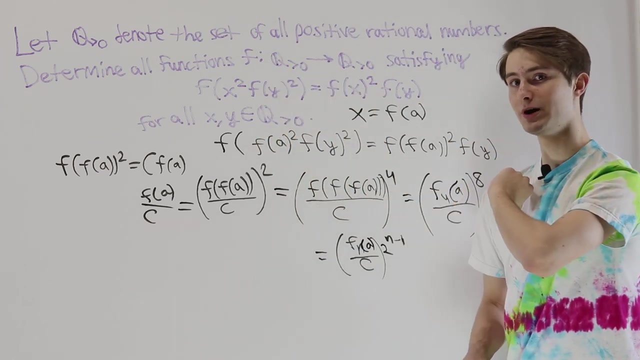 remember that is equal to f of a over c. Now let's think about what this means, Because there's one other condition that we haven't used that much so far, Which is that f goes from positive rational numbers to positive rational numbers, Which means 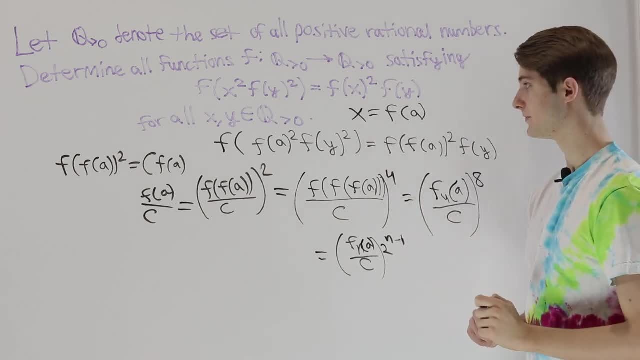 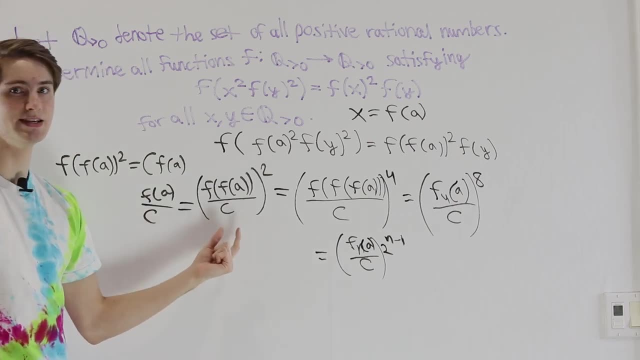 that everything we're looking at right here has to be rational. f of a has to be rational because we know the function maps to positive rational numbers And remember that our constant c that was originally defined as a ratio of two values of our function. 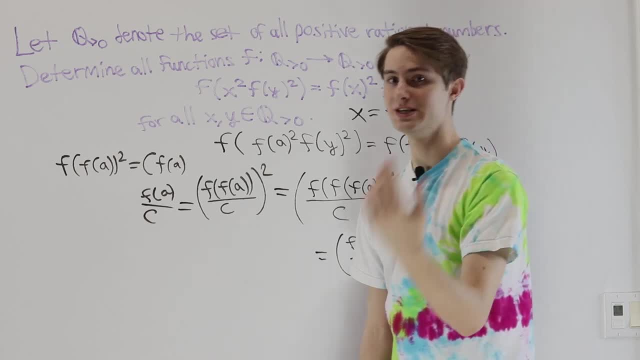 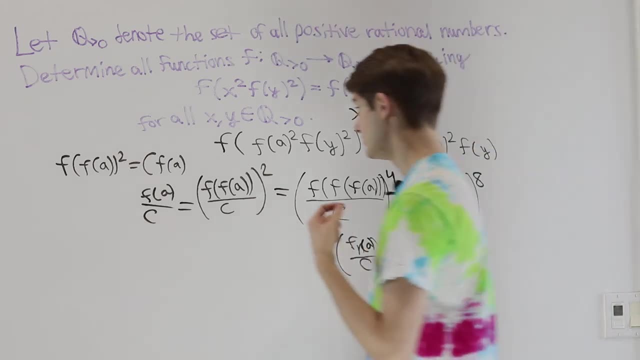 And a rational number divided by a rational number has to be another rational number. So this thing that we have right here- f of a over c- that is rational, And so is what we have down here. It's another rational number raised to some power. 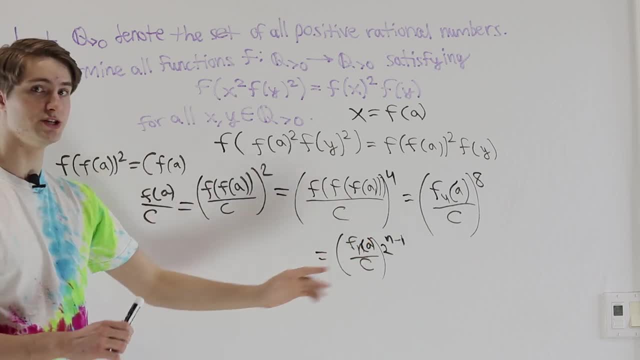 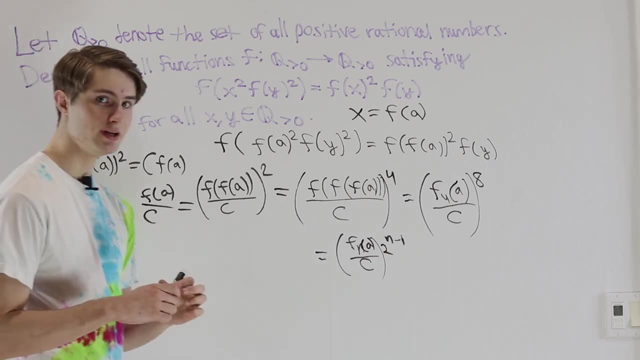 But now we have to think about what does it mean for everything in this equation to be a rational number? Well, we know f of a over c, that's going to have to equal as a rational number some product of prime numbers divided by another product of prime numbers. 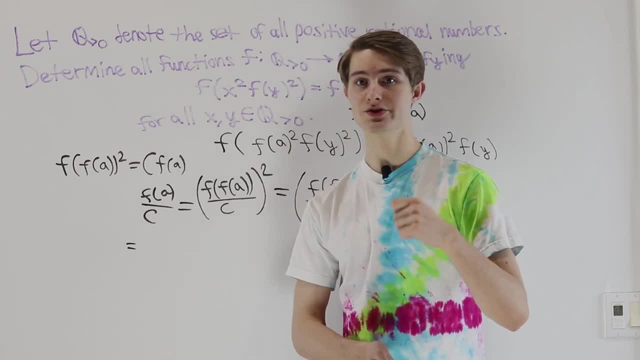 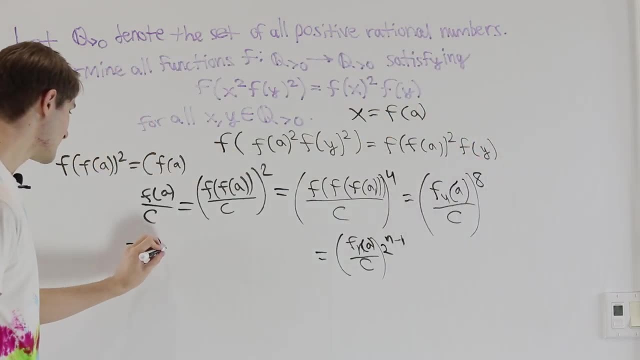 Because we know that rational numbers are a ratio of integers and integers are always made up of primes, So f of a over c. well, that's going to equal some prime p1 to the power of k1, times some prime p2 to the power of k2,. 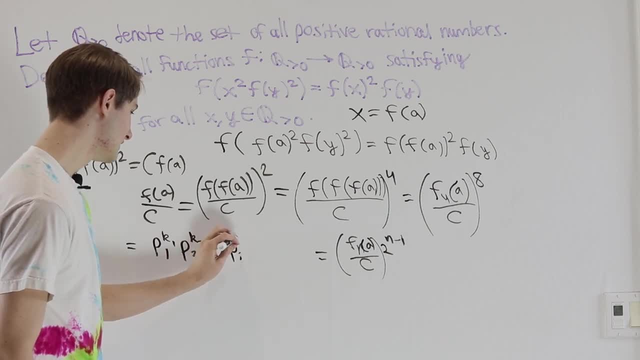 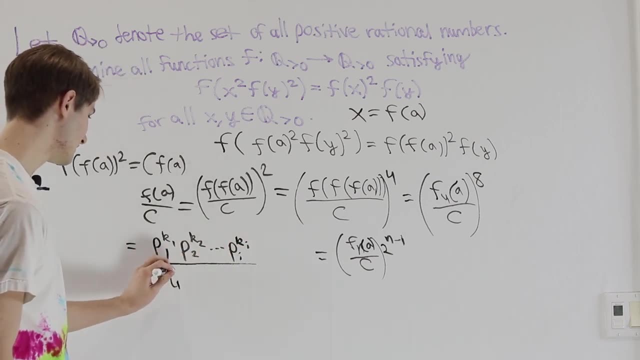 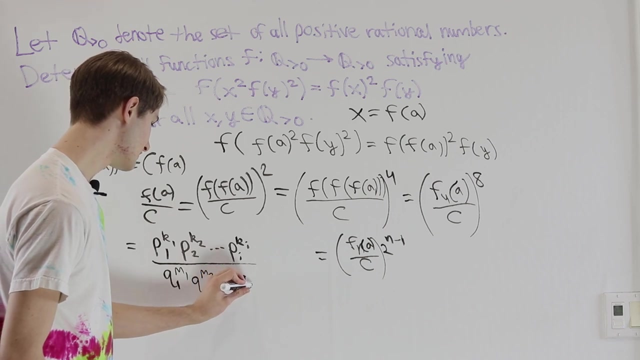 and so on. to prime, for example, pi to the power of ki And that's going to be divided by some prime, q1 to the m1, times q2 to the m2, and so on to qj to the power of mj. 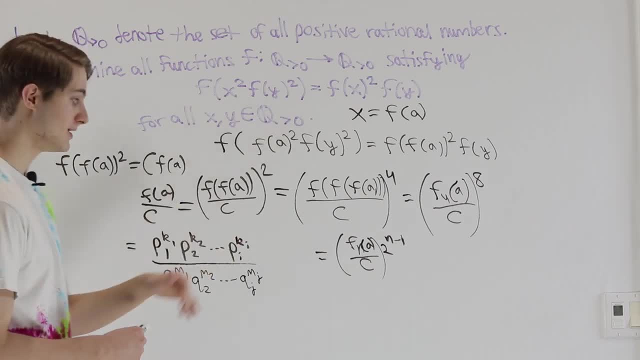 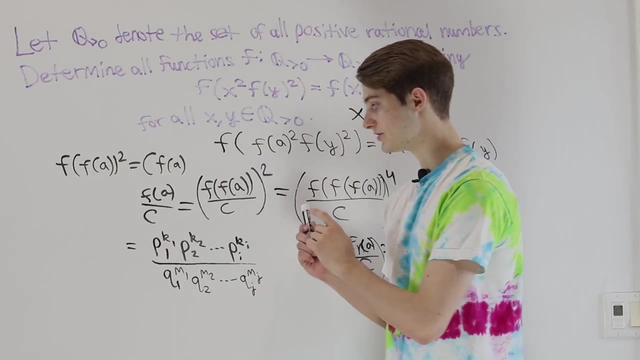 All this is saying is we have primes on the top and primes on the bottom. These aren't going to cancel out, because we'll say: our fraction is in reduced form and all of these powers are finite. But now let's take a look at what we have over here. 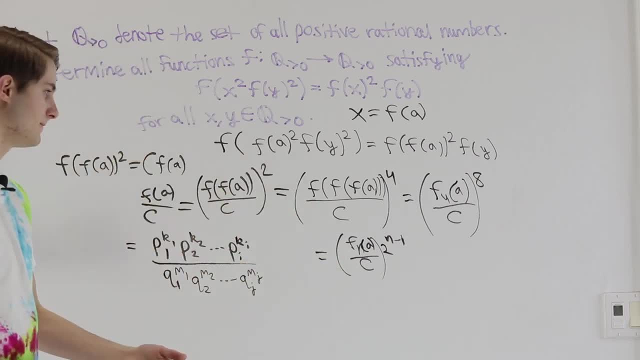 We have f of a over c. that's going to be a rational number, but then raised to the power of 2 to the n-1.. That's pretty big, And what we have to remember is this is true for any value of n. 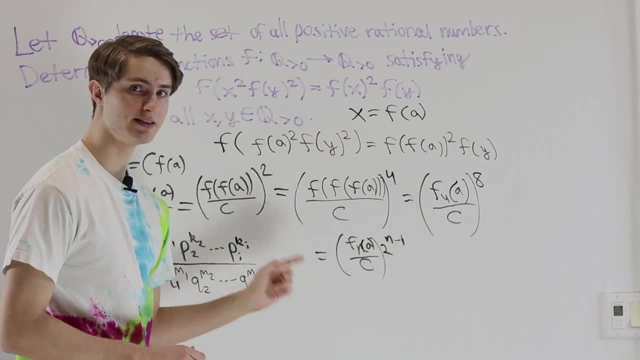 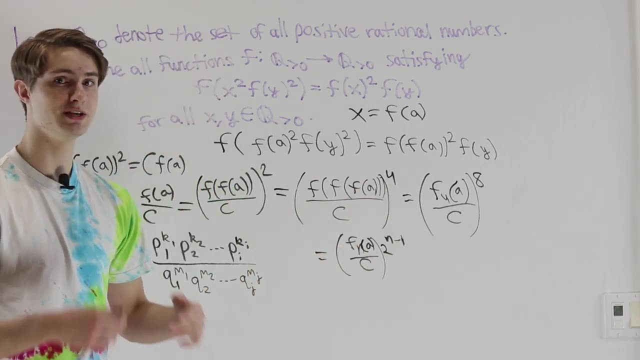 because we can keep iterating this process to make that value arbitrarily large. We can make n as big as we want. So this power could be 512,, it could be 1024,, it could be a billion. We can make it as big as we want. 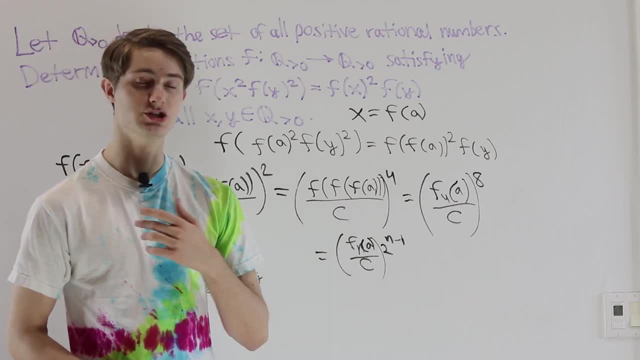 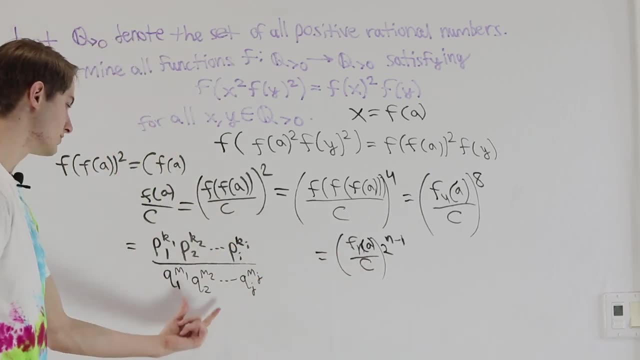 In fact we can make it approach infinity because it can just keep on increasing. But that's a little weird because if this is a rational number in here, it's also going to be a ratio of prime numbers on the top and prime numbers on the bottom. 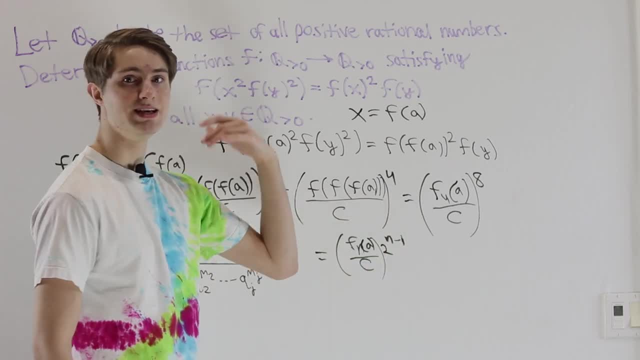 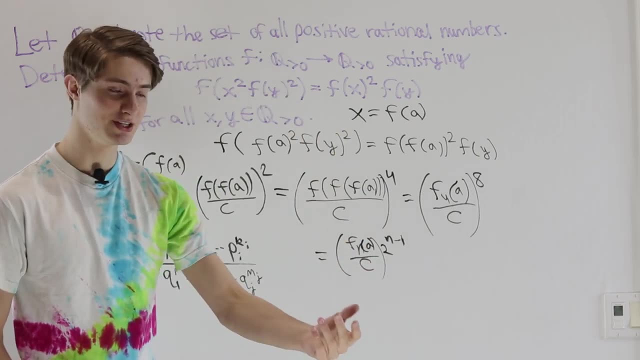 But if this is a fraction and we're raising it to an infinitely increasing power, then the powers of the prime numbers in here are also going to increase infinitely, And if we can just keep making those bigger, well, that's never going to be able to equal. 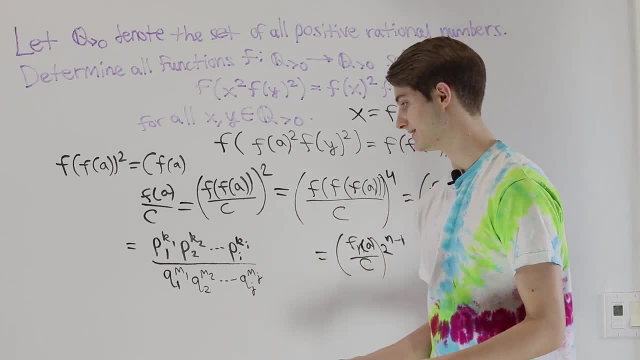 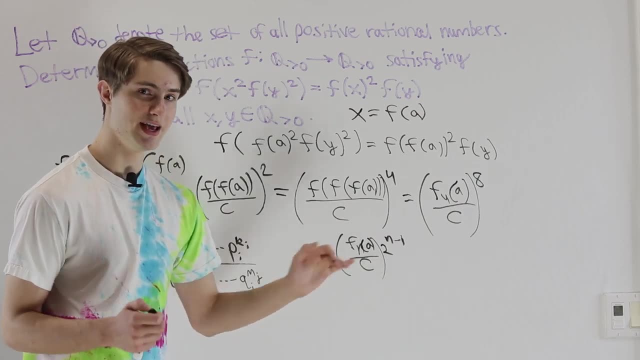 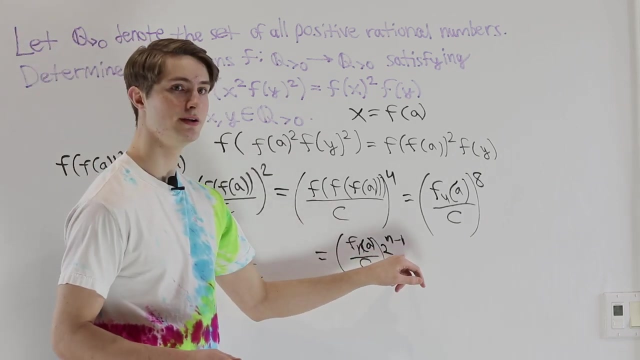 a finite rational number. That just doesn't make any sense. So there's no way that this works when we have a fraction on the inside. Is there any rational number where this would be possible? Well, it has to be one where, when we raise it to a power, 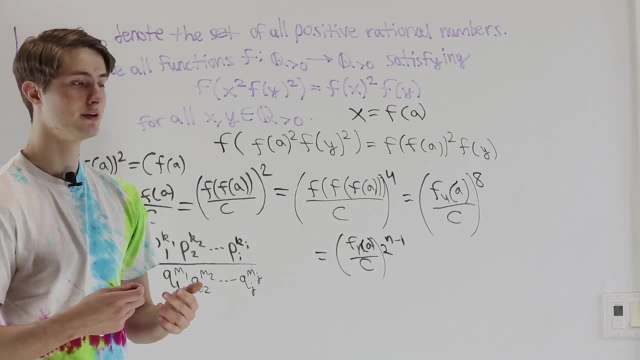 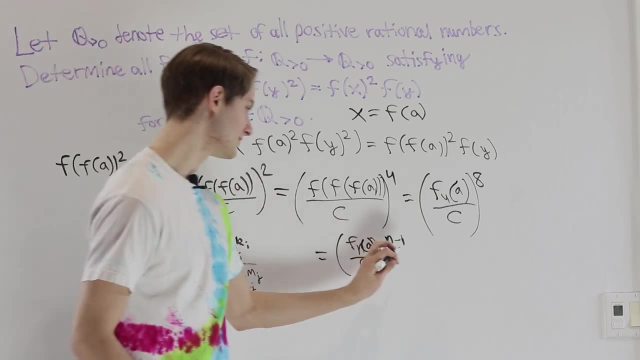 it doesn't keep getting bigger and bigger and bigger. What rational number, when we raise it to a power, doesn't change? Well, there's only one rational number that does that, and it's one Because one is a ratio of no prime numbers. 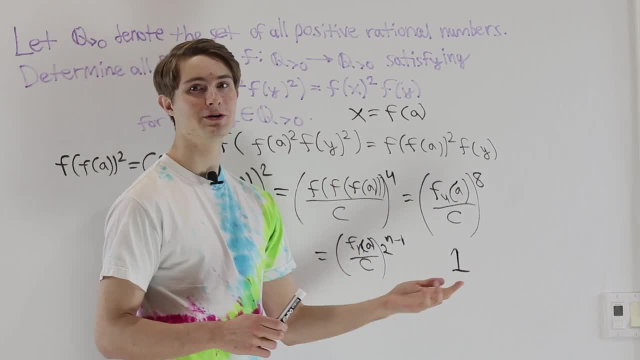 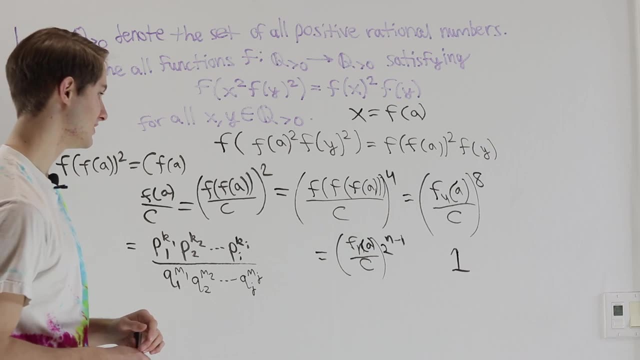 It's an empty product, And one to any power is just going to give us one right back. So the only way that we can avoid those infinitely increasing powers that don't make any sense is by having one as our answer. This function here. 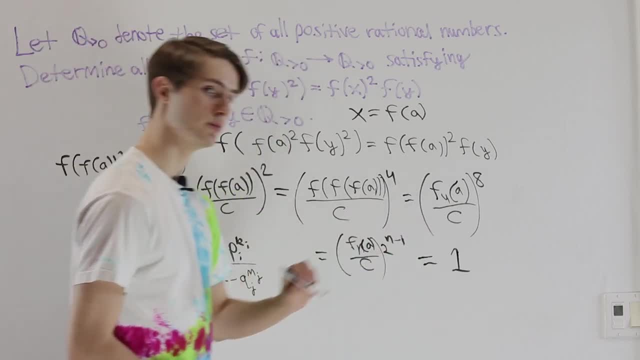 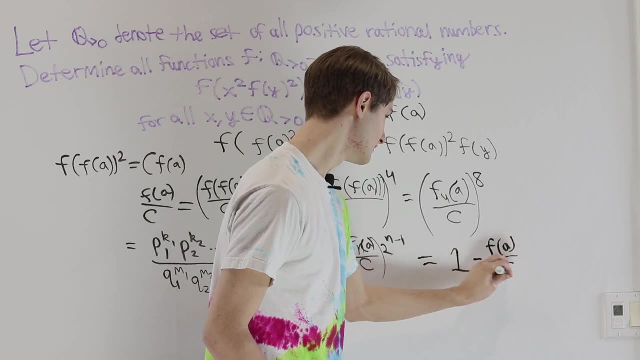 f sub n of a over c, that has to equal one, So that when we raise it to the power it's still one, And therefore we know that f of a over c is also equal to one. So f of a is going to be a constant. 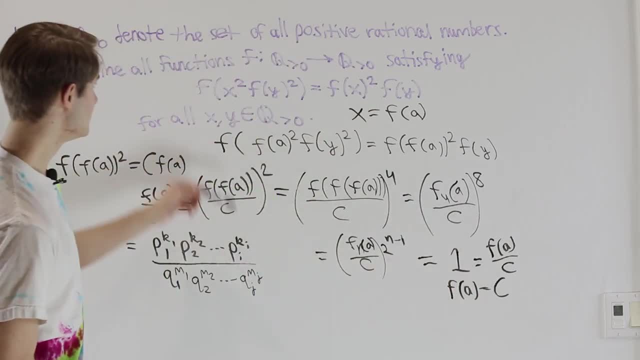 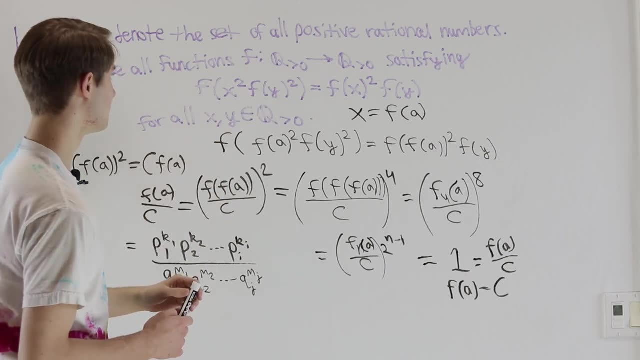 All we have to do now is figure out what that constant is using our good old equation up here. Well, doing that is pretty simple. We can just plug in everything that we see here On the left side f of we don't care what the input is. 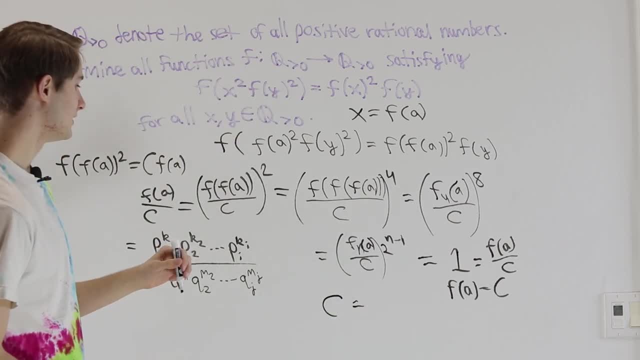 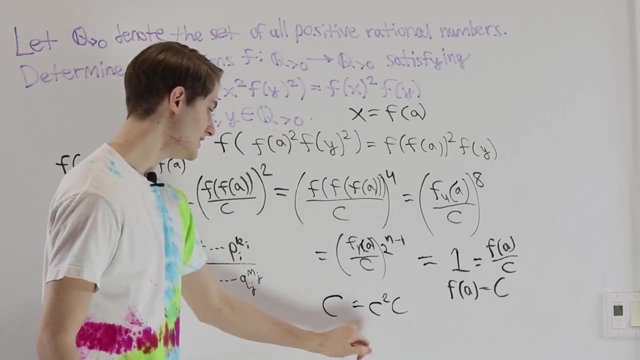 it's going to be c. So on the left side we have c, On the right side we have f. of whatever, that's going to be c squared times another c, Or in other words c equals c, c cubed. 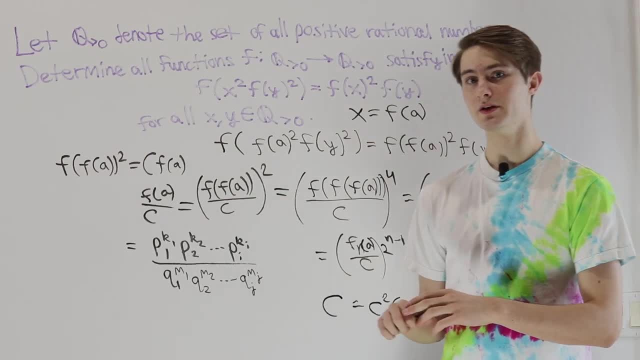 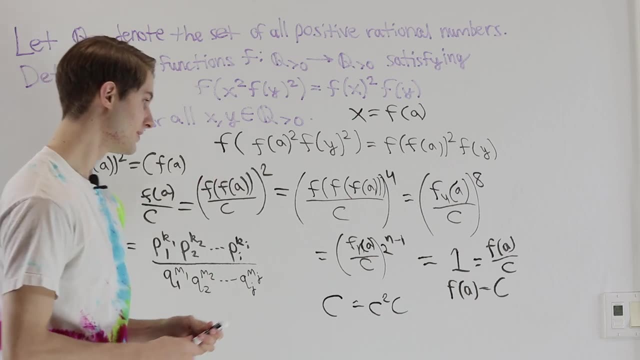 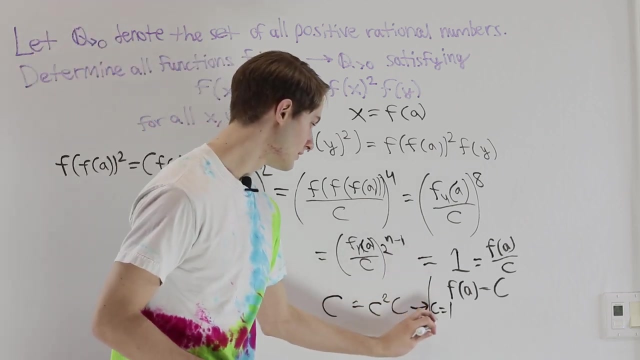 Remember, we're looking at positive rational numbers only. The only positive rational number, where c equals c, cubed is going to be: c equals one And therefore we know our function f of a has to be equal to one. That is the only possible solution. 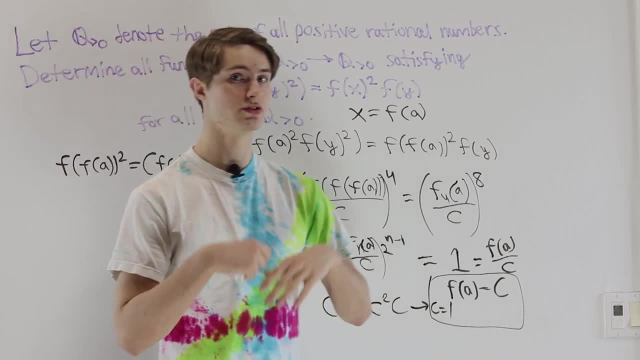 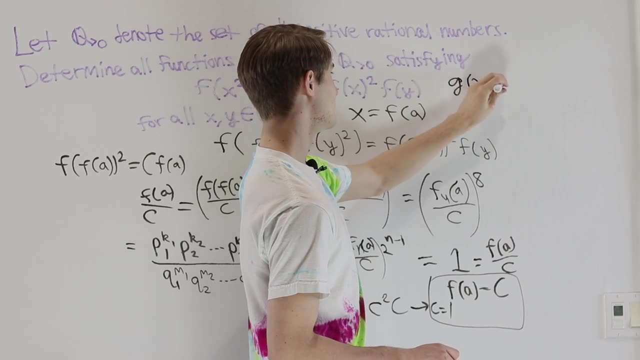 to this function. Now, if we were looking at functions that weren't strictly rational, then there would be other answers. For example, one way to solve this is setting g of x equal to the square root of x. However, that doesn't satisfy the condition. 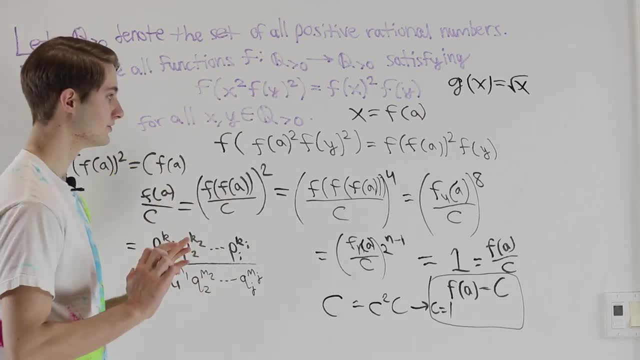 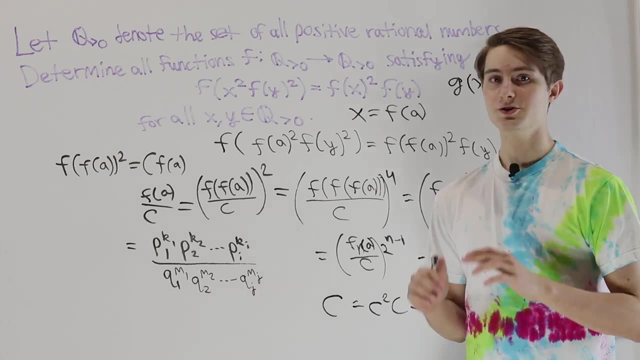 that we're only looking at positive rational numbers. So the way that we got to this answer and the way that you should try to approach a lot of functional equation problems is by starting from the perspective of where can I find symmetry in the problem? 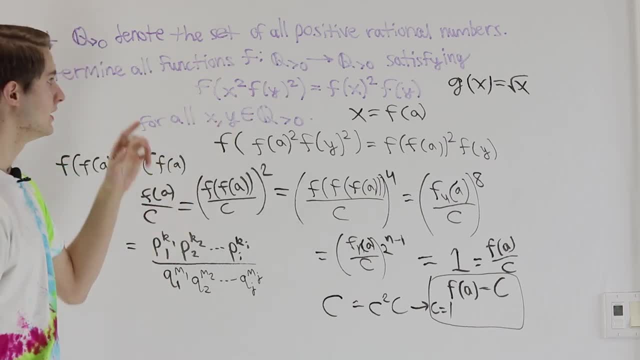 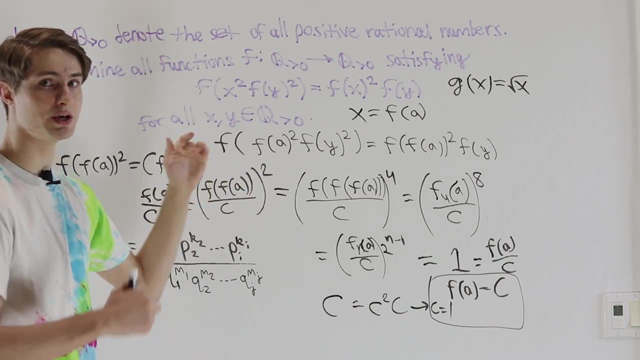 In this case we saw x squared and f of y squared, and just from that we were able to get to a position where we could find something that was symmetric, and then we could play around with the variables. We found another symmetric equation over here. 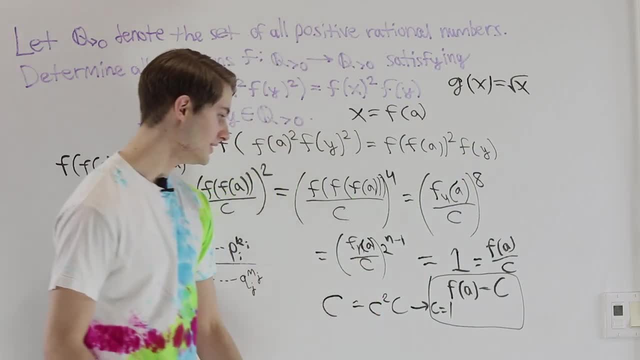 and from that we were able to get all the information that we needed to solve for our answer just like this. 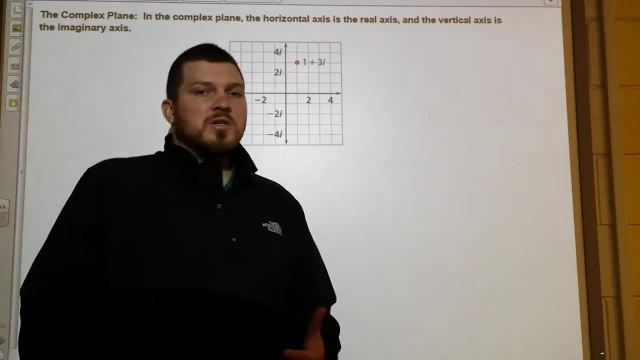 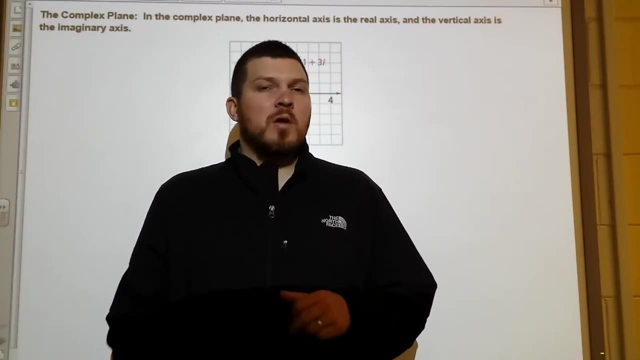 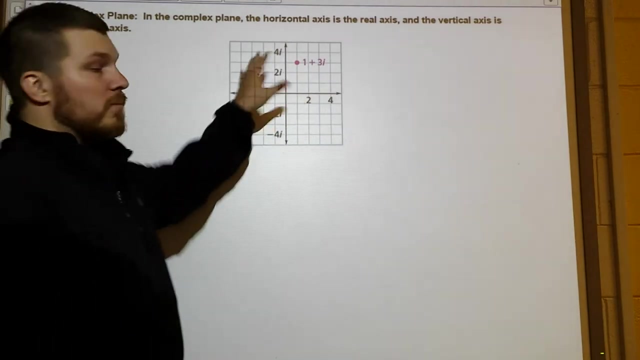 All right. so in this video, what we're doing is talking about finding the magnitude or absolute value of a complex number, But first we need to figure out what does the absolute value of a complex number even mean? So let's look at the picture, So the complex plane. it looks a lot. 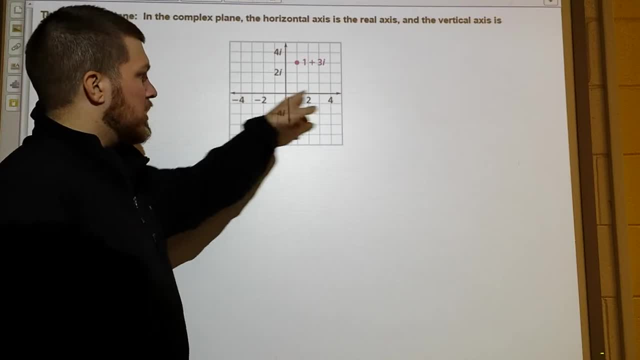 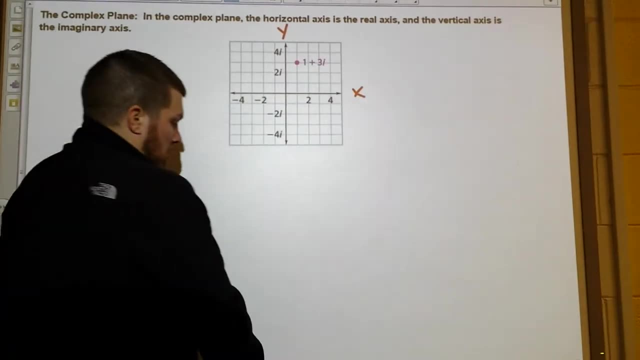 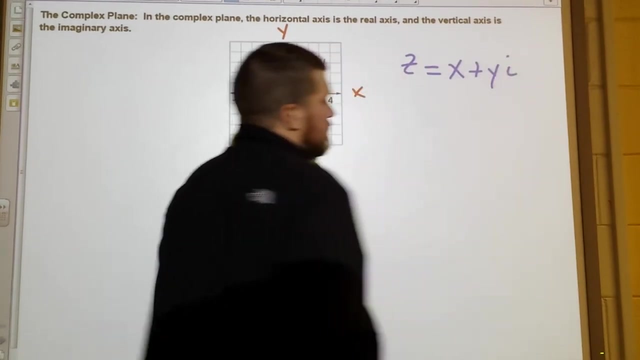 like the coordinate plane that we're all familiar with. In the coordinate plane, we have the x-axis, which goes from left to right. We have the y-axis which goes up and down. Well, remember our complex number, which we typically call z, is the same thing as x plus yi. okay, So in the 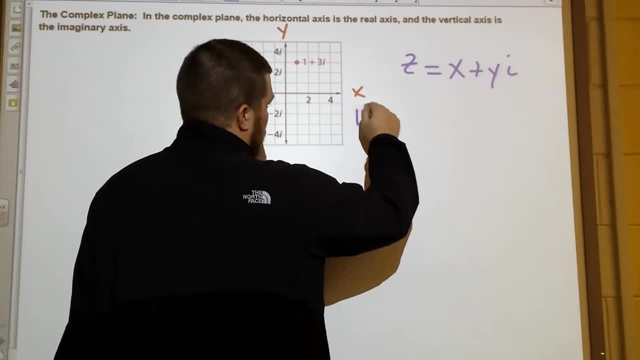 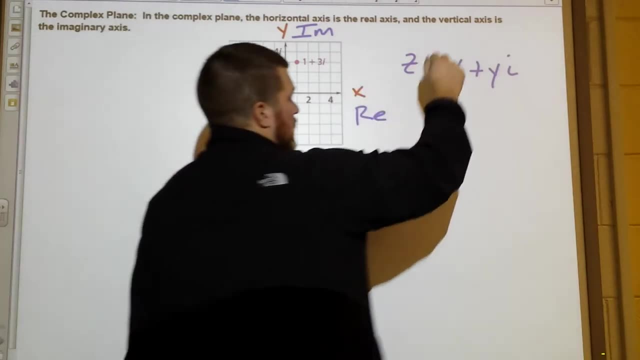 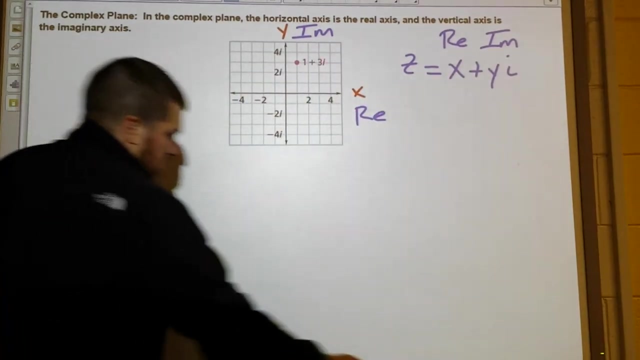 complex plane. our x-axis is going to become the real axis and our y-axis is going to become the imaginary axis, because our x is the real part, our y is the imaginary part. okay, So, for instance, the complex number 1 plus 3i.